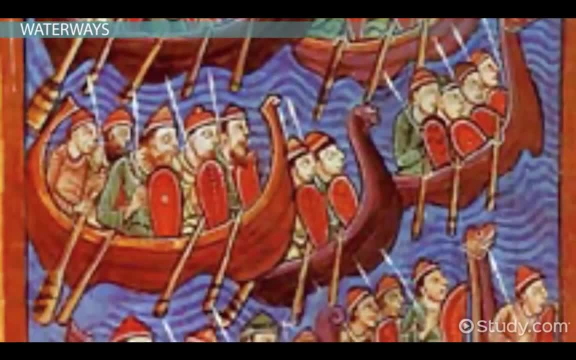 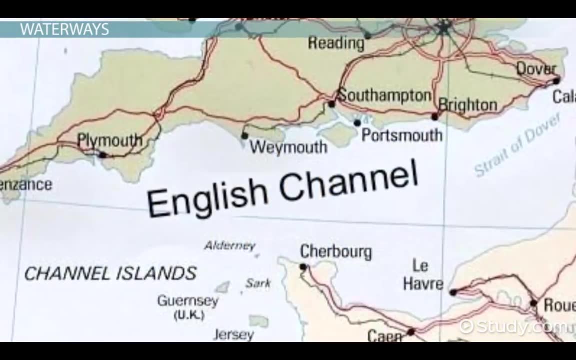 too. The Vikings could have never launched their raids without the Baltic and the North Seas, and a part of the North Sea called the English Channel kept Britain free from invasion for most of history. However, it's not just saltwater that's important to Europe. Many rivers. 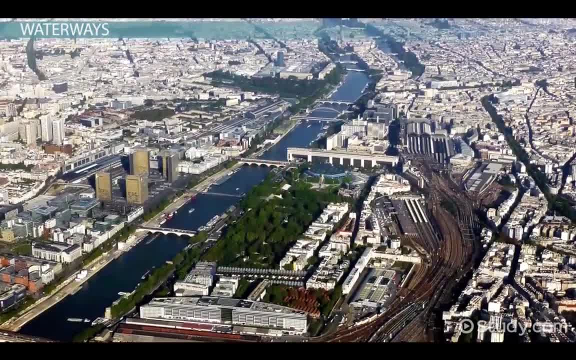 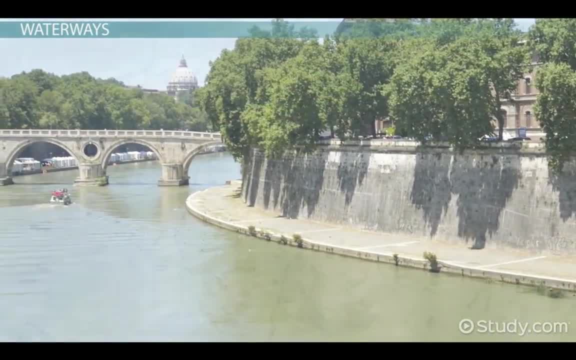 cross the continent. Some of these you may have already heard of, because they flow through big cities like the Seine in Paris or the Tiber in Rome. One of the biggest rivers in Europe has served as a border for some of its greatest cities. The Baltic Sea is one of the most important. 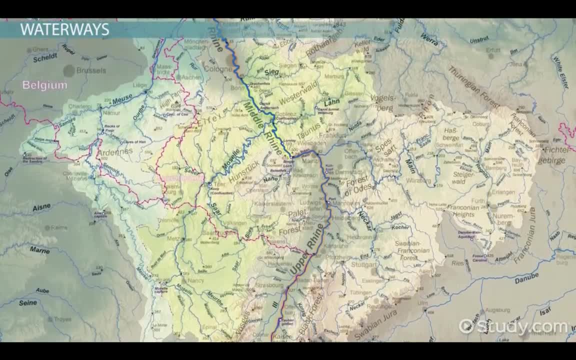 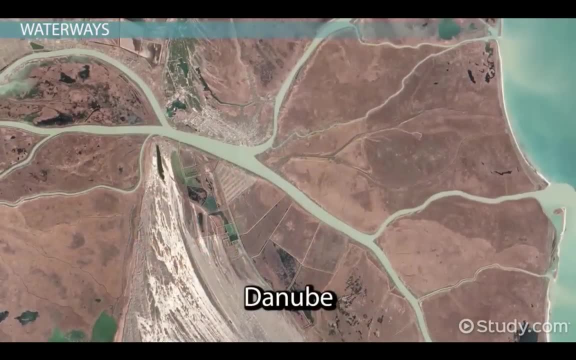 empires. Historically, France and Germany, two of Europe's most important countries, have had the Rhine as their boundary. On the other hand, the Danube serves as a connector between many of Europe's cultures in the southeast, allowing for better communication. Both rivers, as well as 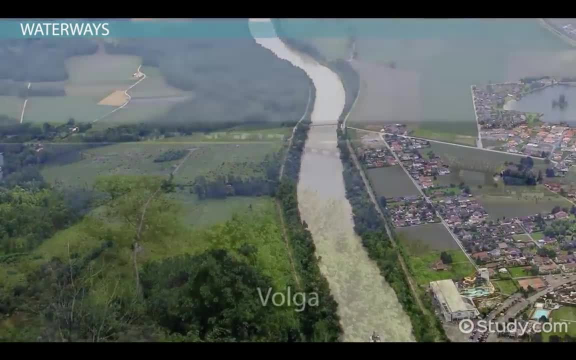 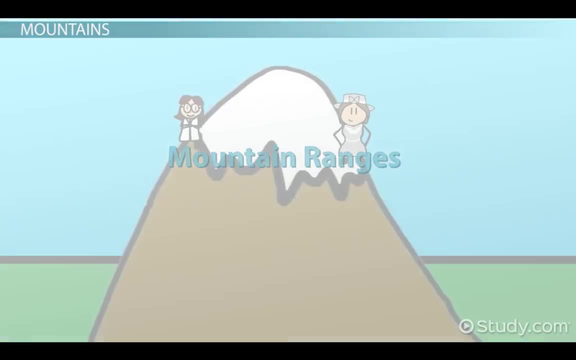 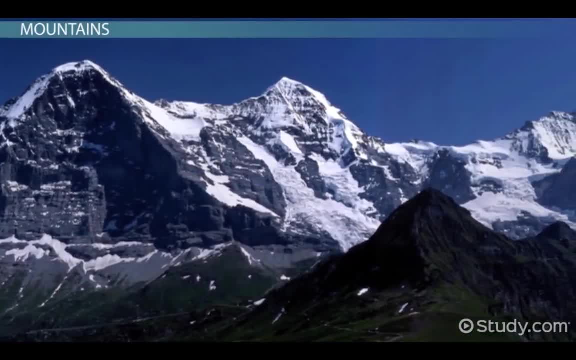 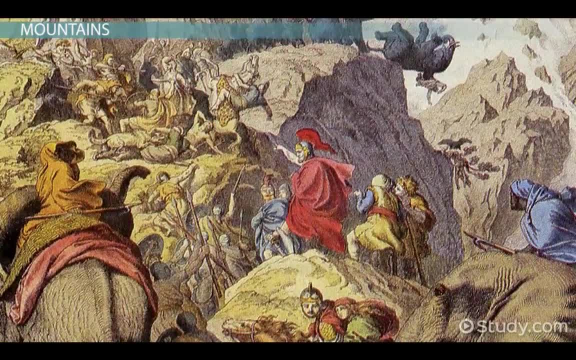 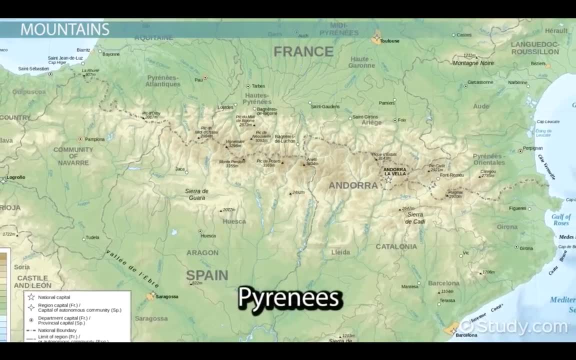 of its history, although invaders such as Hannibal and Napoleon often crossed them. Other mountain ranges in Europe also serve as boundaries, including the Pyrenees between France and Spain and the Carpathians that separate Romania from much of the rest of Europe. 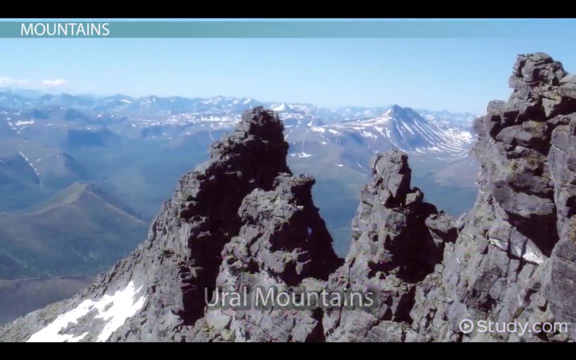 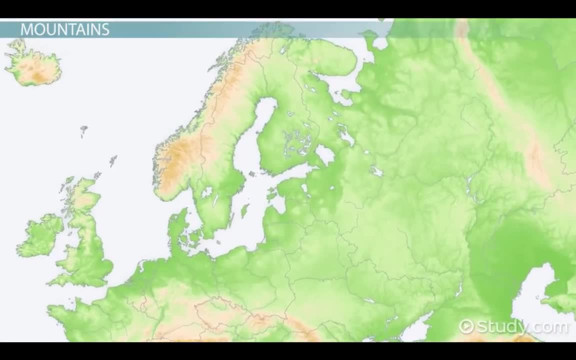 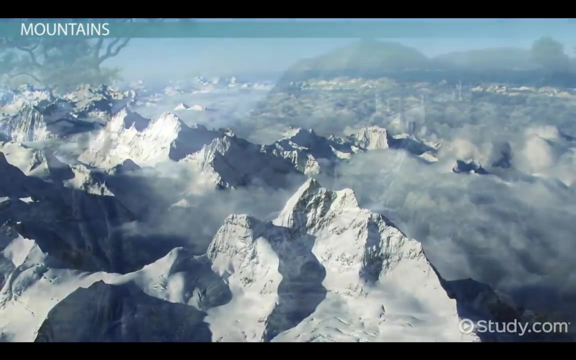 In fact, the Ural Mountains act as a boundary for Europe itself. Anything east of them is considered part of Asia, while anything west is European. Still other mountains are worthy of note because of how they've historically affected the people who live there. In places like Greece and Norway, mountainous terrain meant that people often found 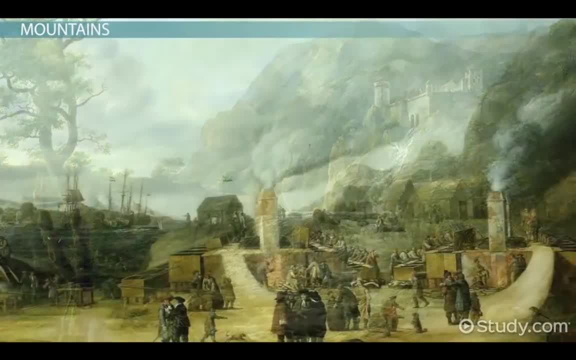 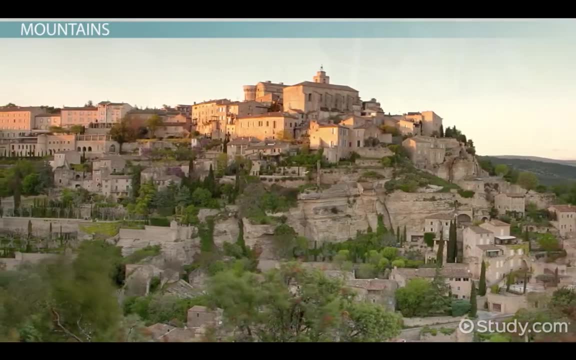 themselves fishing instead of farming, using what fields they could on more valuable crops. Likewise, the low hills of southern France and Italy lent themselves to growing grapes for wine, something both countries are still known for producing. Yet it is not just land that determines. 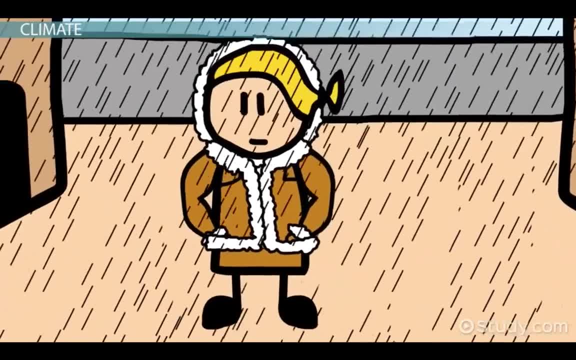 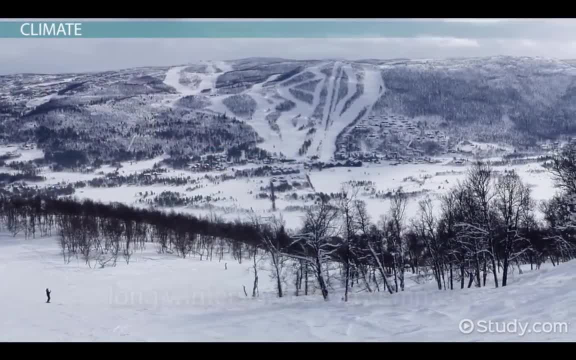 how people can use a given area. Climate matters a great deal too. Within Europe, the climate varies dramatically. In the far north, including places like Norway and Sweden, people have long winters and short summers. On the other hand, in Italy and Greece, people have the exact opposite.